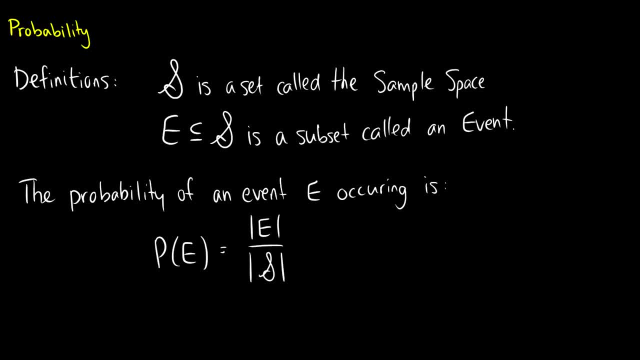 I don't like writing that R out every time, so I take it out. Some people may confuse it with the power set, but again, if I use the power set, I use that P for the power set, So there is a distinction here. This is the probability and it's the number of elements in E divided by the. 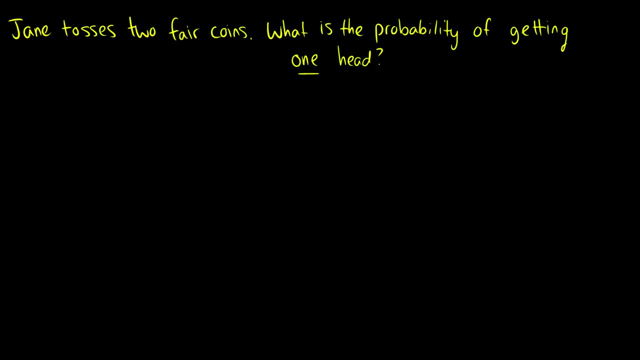 number of elements in the sample space. So that's basic definitions. Let's do a problem right away. Jane tosses two fair coins. What is the probability of a fair coin? Jane tosses two fair coins. What is the probability of a fair coin? 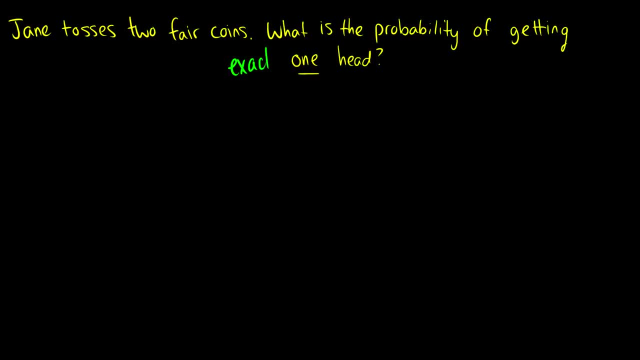 The probability of getting one head. This is exactly one head, So I'll make this super clear: Exactly one head. Let's write out a sample space. So how many ways can she toss two coins? Well, in her first toss she could get the first coin as a head and the second coin as a head. 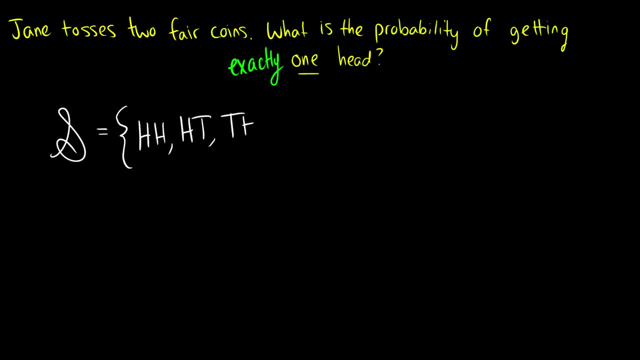 The first coin is a head and the second is a tails. The first is a tails, the second is a head, or the first is a tails and the second is a tails, So there's four possible ways of throwing it. Now our event E is going to be the case where she gets either a head and a tail or a tail, and 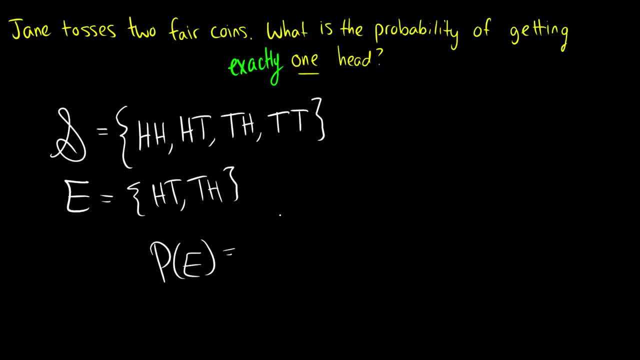 a head. So the probability of that event happening is the number of elements in our event over the number of elements in our sample space. So this is going to be two divided by four, which is one half. So it's a nice simple problem. Now there's something more we can do with this. 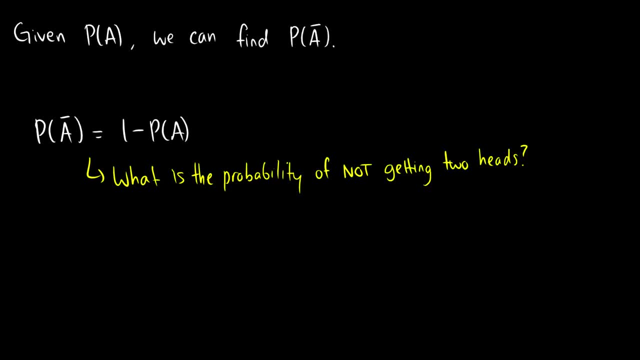 If we get the probability of a, we can find the probability of not a or a complement. So the complement is everything that is not in that set, And this is going to be equal to one minus the probability of a. We'll prove this in the next video. 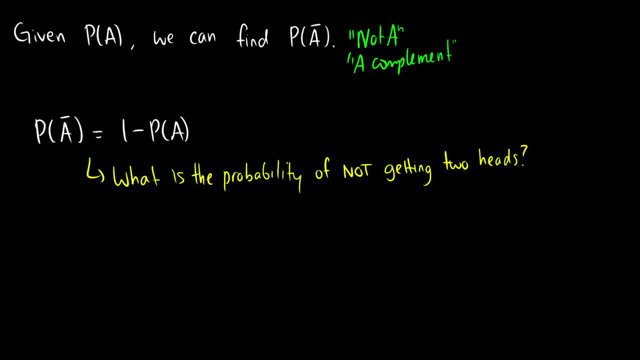 So what is the probability of not getting two heads? So let's find the probability of two heads. So this is equal to the case where we get h, h over the sample space. So this is going to be one. fourth, Now, the probability of not getting two heads is going to be one. 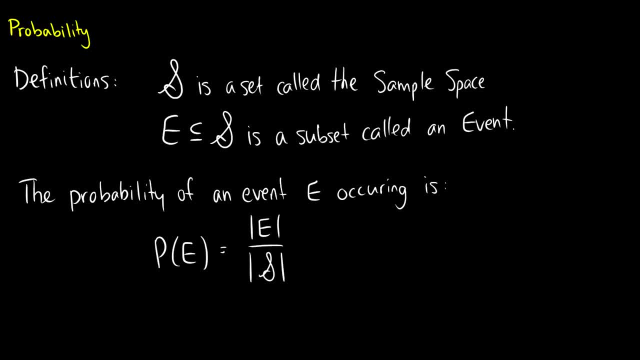 I don't like writing that R out every time, so I take it out. Some people may confuse it with the power set, but again, if I use the power set, I use that P for the power set, So there is a distinction here. This is the probability and it's the number of elements in E divided by the. 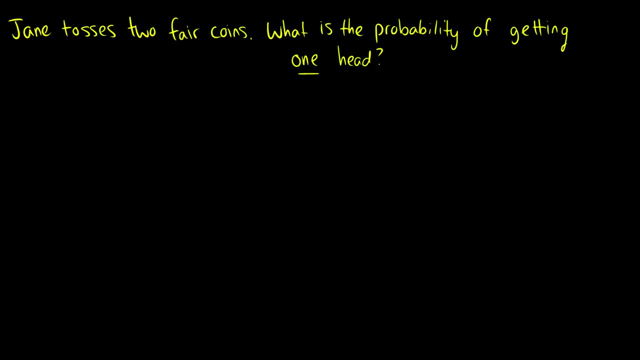 number of elements in the sample space. So that's basic definitions. Let's do a problem right away. Jane tosses two fair coins. What is the probability of a fair coin? Jane tosses two fair coins. What is the probability of a fair coin? 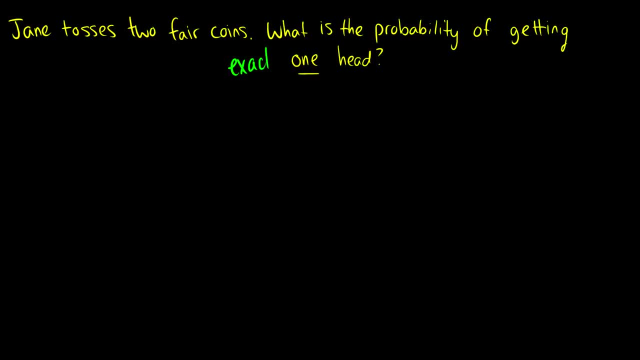 The probability of getting one head. This is exactly one head, So I'll make this super clear: Exactly one head. Let's write out a sample space. So how many ways can she toss two coins? Well, in her first toss she could get the first coin as a head and the second coin as a head. 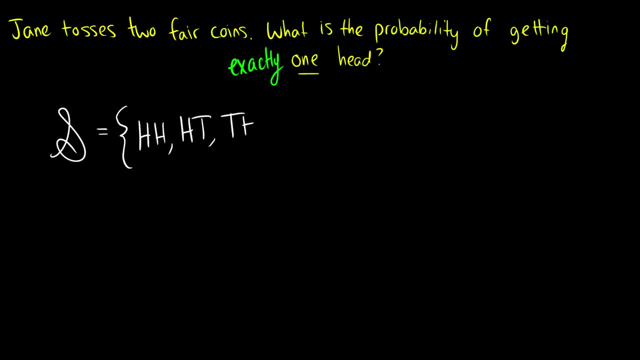 The first coin is a head and the second is a tails. The first is a tails, the second is a head, or the first is a tails and the second is a tails, So there's four possible ways of throwing it. Now our event E is going to be the case where she gets either a head and a tail or a tail, and 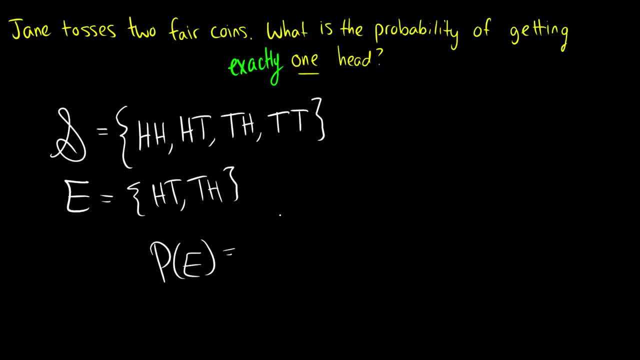 a head. So the probability of that event happening is the number of elements in our event over the number of elements in our sample space. So this is going to be two divided by four, which is one half. So it's a nice simple problem. Now there's something more we can do with this. 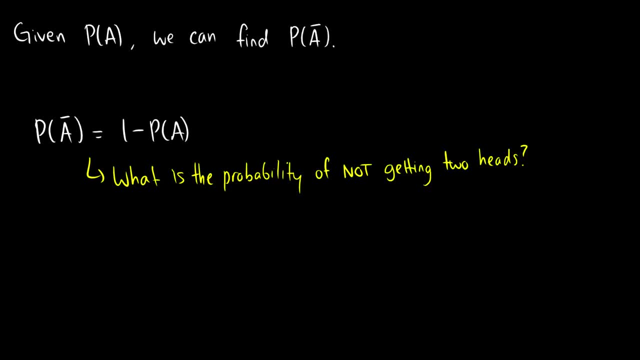 If we get the probability of a, we can find the probability of not a or a complement. So the complement is everything that is not in that set, And this is going to be equal to one minus the probability of a. We'll prove this in the next video. 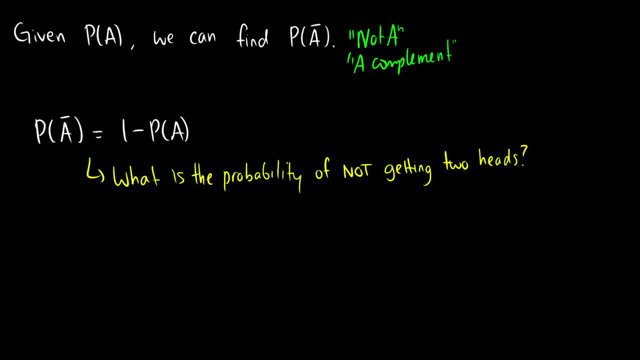 So what is the probability of not getting two heads? So let's find the probability of two heads. So this is equal to the case where we get h, h over the sample space. So this is going to be one. fourth, Now, the probability of not getting two heads is going to be one. 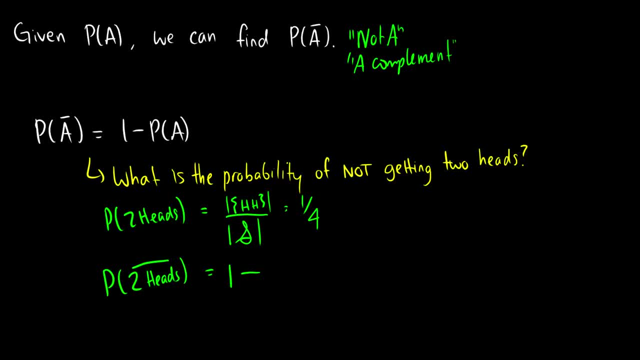 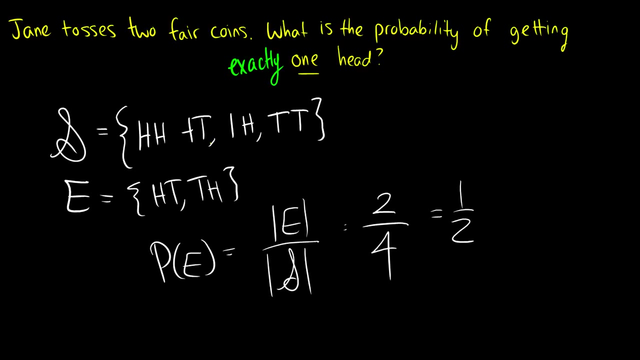 minus the probability of getting two heads, which is going to equal one, minus one fourth, which is just equal to three fourths, And we could do this with the sample space. So the probability of not getting two heads. well, that's going to be this situation. Whoa, that was weird. That's going to 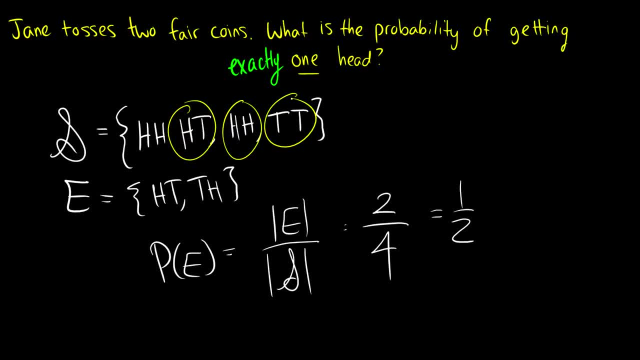 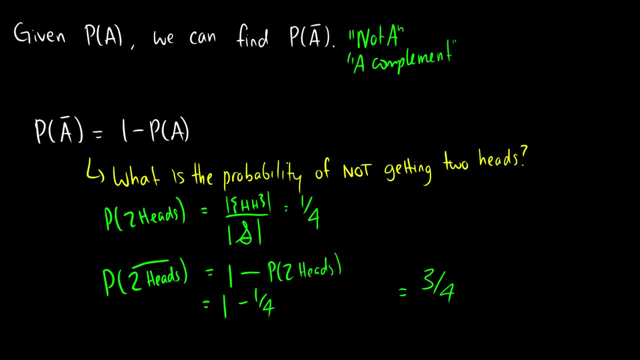 be this situation. So we're going to get two heads. So we're going to get one minus the probability of situation, this situation and this situation, which is 3 out of 4.. So it works. with our intuition and by using a simple example, we can verify this. So that's kind of nice. 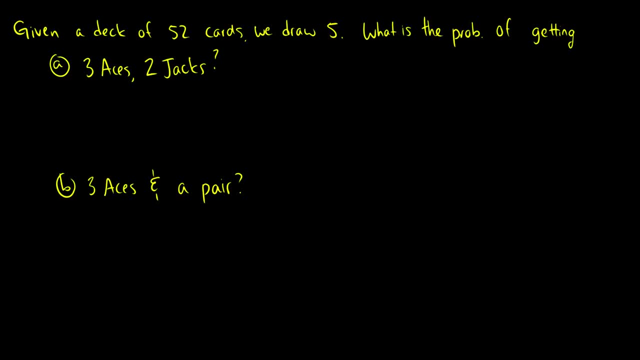 We can find complements. Now let's do some combinatorics problem. This is why I did the counting review. So, given a deck of 52 cards, we draw 5.. Now, what is the probability of getting 3 aces and 2 jacks? Well, this is going to be this event. so what is the event? 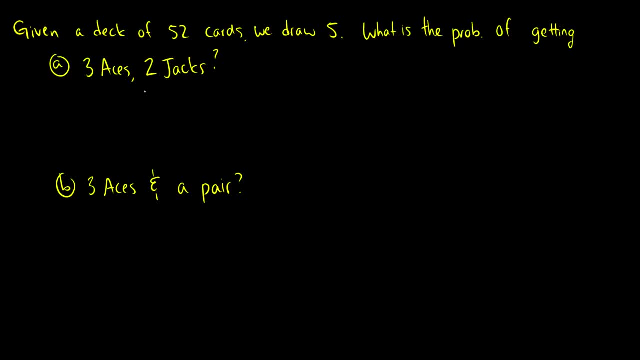 of getting 3 aces and 2 jacks. Well, there's 4 aces. so out of the 4 aces, we're going to choose 3 of them, and out of the 4 jacks, we're going to choose 2 of them. So that's. 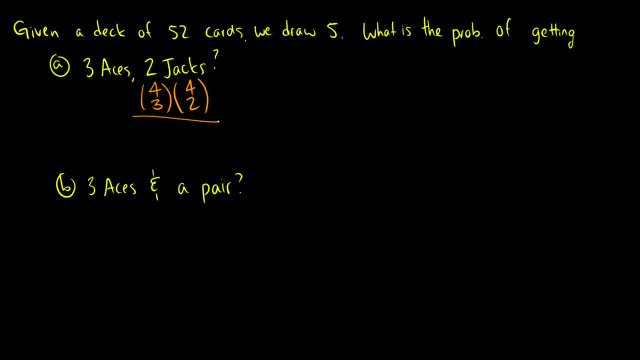 the event E happening. Now. what is the sample space? Well, the sample space is all the possible combinations of cards we can draw. so that's going to be 3 aces and 2 jacks. So that's 52, choose 3.. So this is 4, choose 3, times 4, choose 2, over 52, choose- sorry, this. 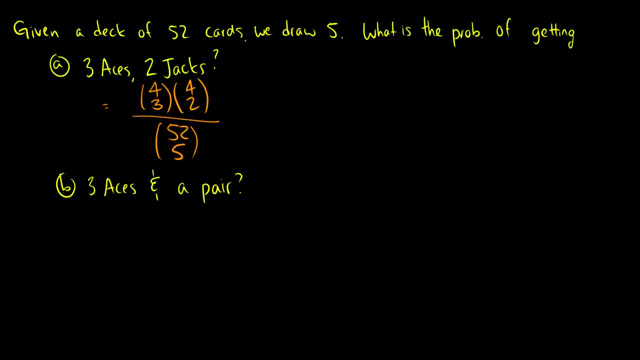 is 52, choose 5, because we chose 5 cards, So it's over 52,. choose 5, because, out of 52 cards, we drew 5 of them. What about 3 aces in a pair? Well, again, this is going. 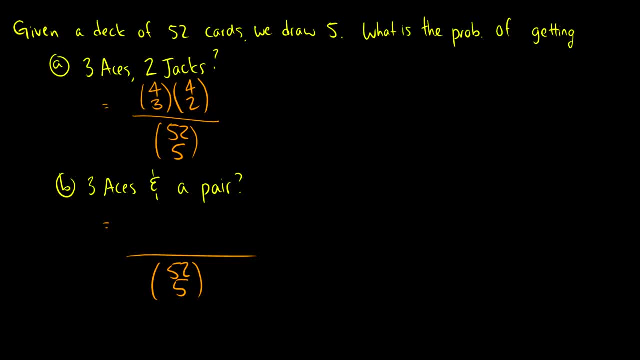 to be something over 52, choose 5.. So 3 aces is going to be something over 52, choose 5.. So 3 aces is going to be something over 52, choose 5.. So 3 aces is going to be something. 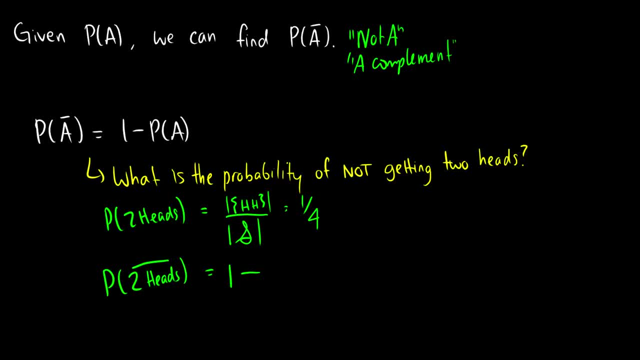 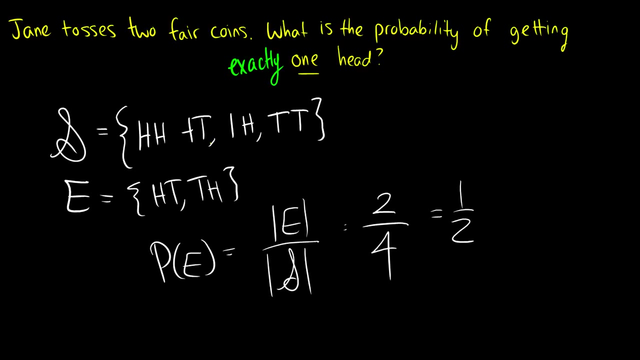 minus the probability of getting two heads, which is going to equal one, minus one fourth, which is just equal to three fourths, And we could do this with the sample space. So the probability of not getting two heads. well, that's going to be this situation. Whoa, that was weird. That's going to 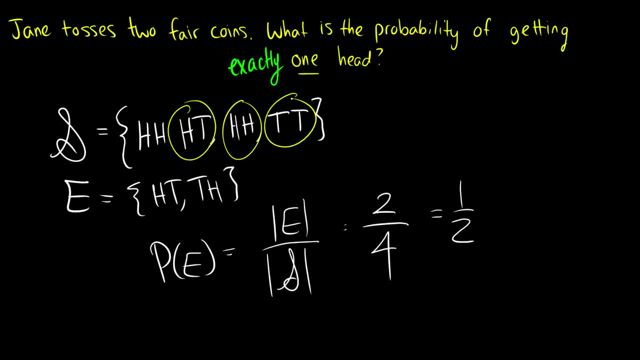 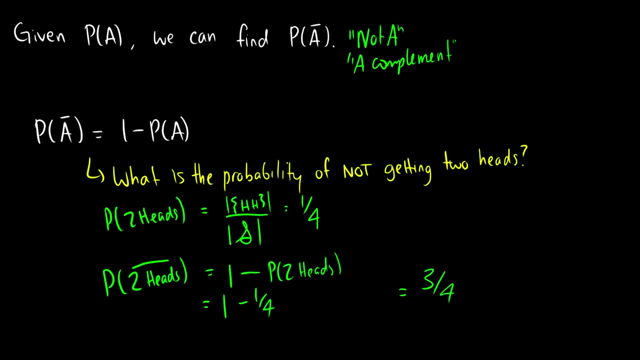 be this situation, So the probability of not getting two heads is going to be one minus one fifth. So everything is equal to one fourth, which is equal to one fourth. So this leads to two heads plus two heads basically. So why are we getting two heads here and only two heads? 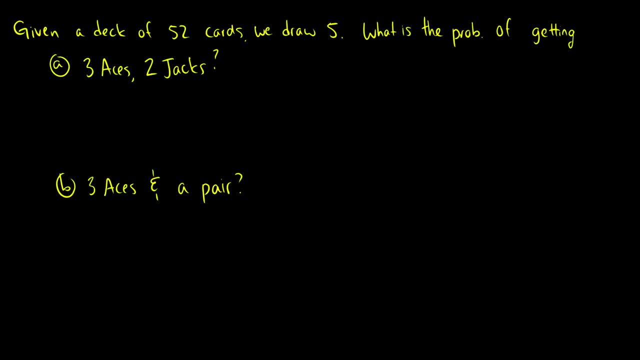 Because, once again, we're only going to get in this situation. In this situation, this situation and this situation. we're just a three out of four. So it works with our intuition and by using a simple example we can verify this. So that's kind of nice. We can find tease. 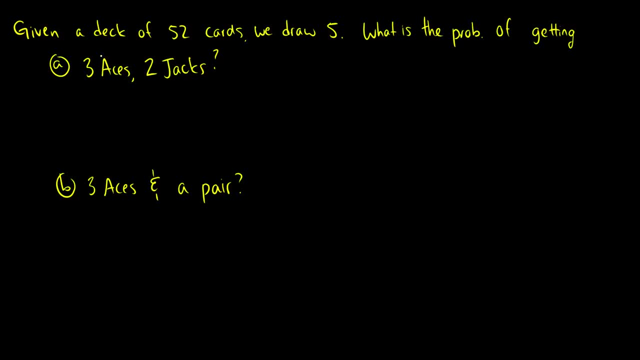 this is going to be this event. so what is the event of getting three aces and two jacks? Well, there's four aces. so, out of the four aces, we're going to choose three of them, and out of the four jacks, we're going to choose: 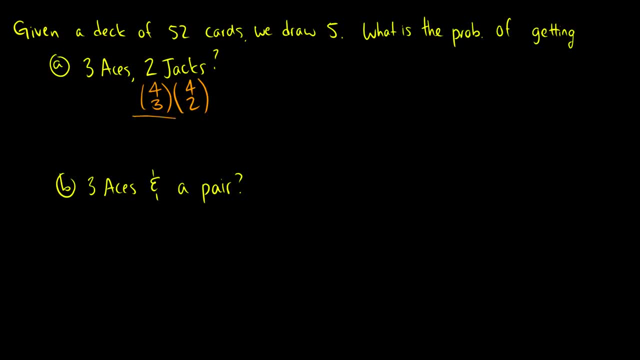 two of them. So that's the event E happening Now. what is the sample space? Well, the sample space is all the possible combinations of cards we can draw. so that's going to be 52 choose three. So this is four choose three. 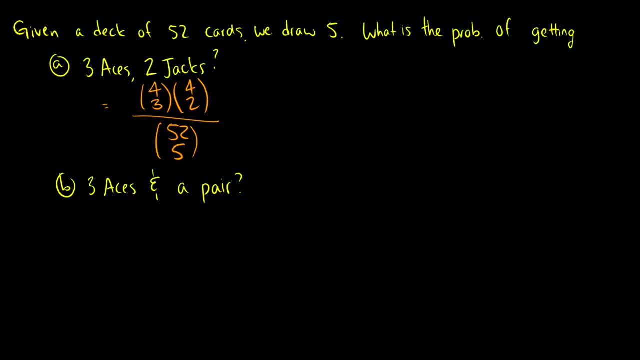 times four. choose two over 52. choose- sorry, this is 52. choose five because we chose five cards, So that's over 52. choose five because out of 52 cards we drew five of them. What about 3 aces in a pair? 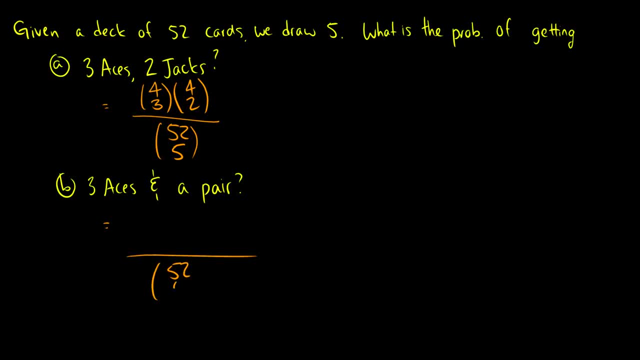 Well, again, this is going to be something over 52. choose five, so three aces is going to be out of four aces we choose. well, a game. it's going to be something over 52. choose five, so three aces is going to be out of four aces we choose. 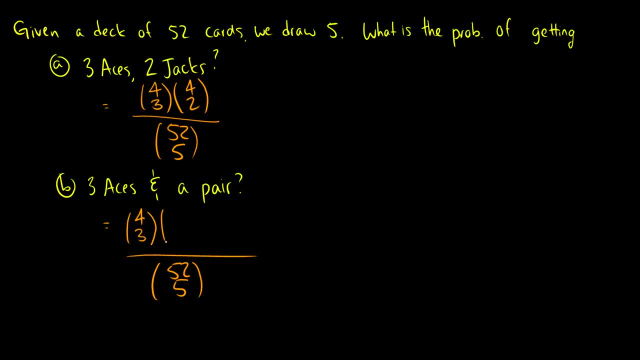 three Now and a pair. Well okay, so there's aces through tens, jacks, queens and kings. We can't choose aces. so there's 12 other suits or there's 12 other cards types that we can pick. 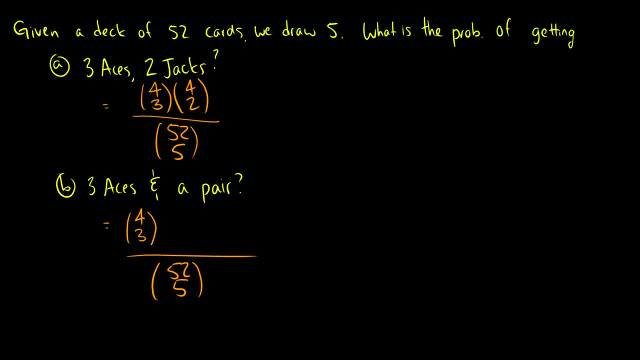 over 52, choose 5.. So 3 aces is going to be something overなんです and we're going 12, so whichever one we chose, if we chose a 4, then we have to choose 2 of those 4 cards. 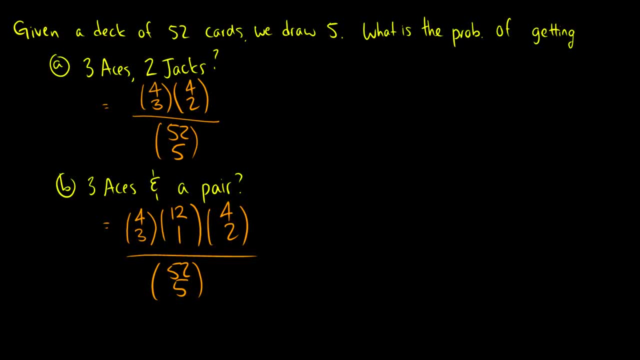 And if we picked a 6, then we'd have to choose 2 of those 6s. Or if we chose a jack, we'd have to choose 2 of those jacks. So this is going to be 4. choose 3 aces times 12. choose 1 number or. 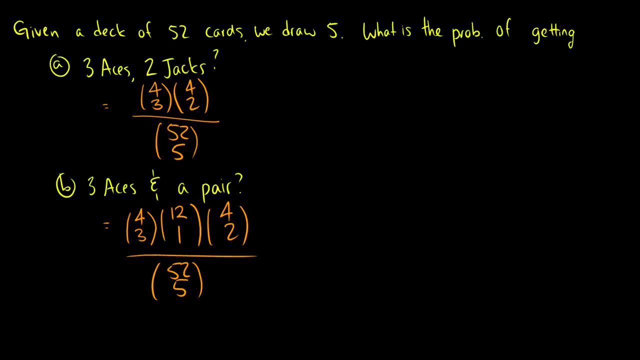 face cards: times 4: choose 2, which is 2 out of those 4 cards that we picked out of the 12. And this is all over 52. choose 5, because we picked, because that's our sample space. 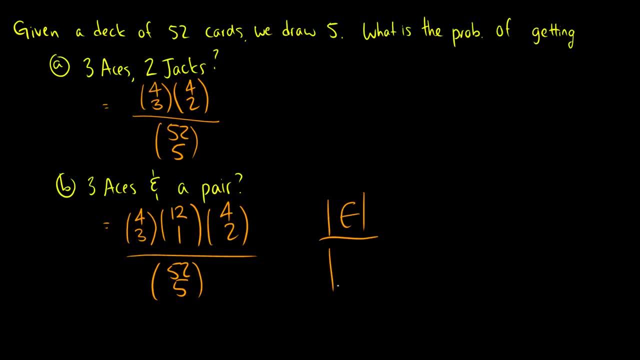 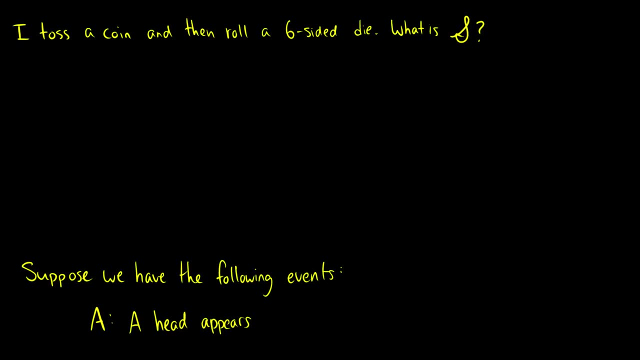 So this is just the probability of an event, or the number of elements in an event over the number of elements in the sample space. So make sure I don't have another question there. Here is Here's another question. I toss a coin and then I roll a 6-sided die. What is the sample space? 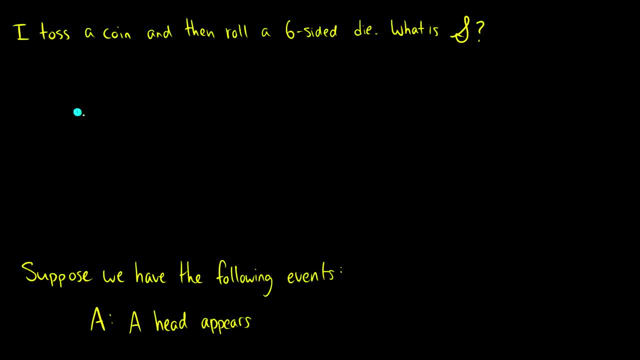 Well, okay, Our first move: we can either pick heads or we can pick tails. Then after we're going to roll a 6-sided die, So you might pick a 1,, you might get a 2,, you might get a 3,, you might get a 4.. 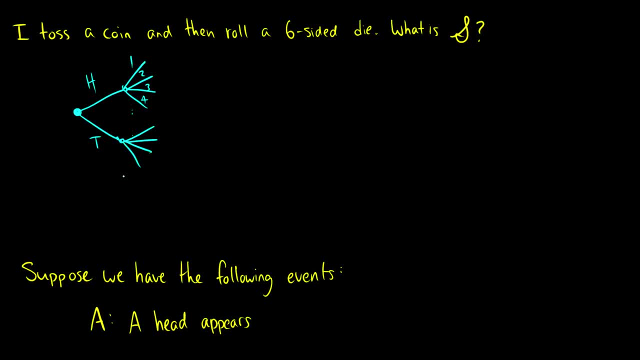 And so on, And same with tails. So that's the same thing. So what we get is, at the end of each of these branches we get a pair, So heads 1, heads 2, heads 3. And this goes all the way down to tails 1, through tails 6.. 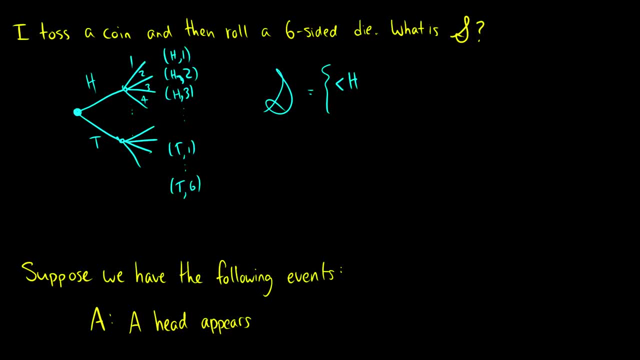 So our sample space is going to be the set of heads 1,, heads 2, and this goes all the way up to heads 6.. And then our next one will be tails 1, all the way up to tails 6.. 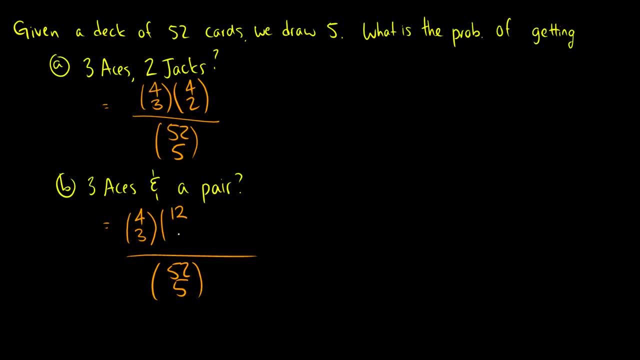 from. There's 12 other number or face cards and we're going to pick one of them And then out of those 12, so whichever one we chose, if we chose a four, then we have to choose two of those four. 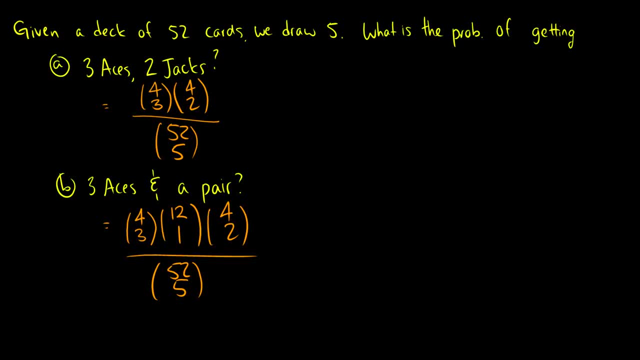 cards, And if we picked a six, then we'd have to choose two of those sixes. Or if we chose a jack, we'd have to choose two of those jacks. So this is going to be four. choose three aces. 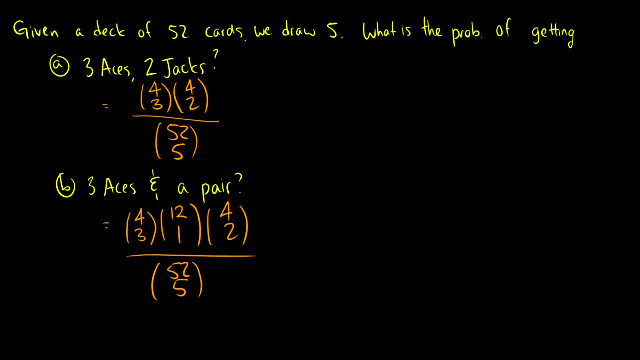 times 12, choose one number or face cards. times four, choose two, which is two out of those four cards that we picked out of the 12. And this is all over 52. choose five because we picked, because that's our sample space. So this is just the probability of an event or the number of elements in an event. 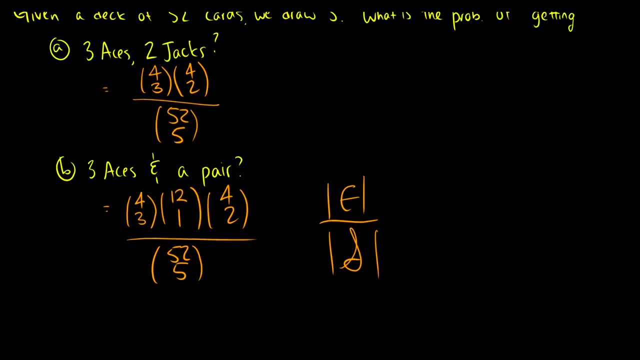 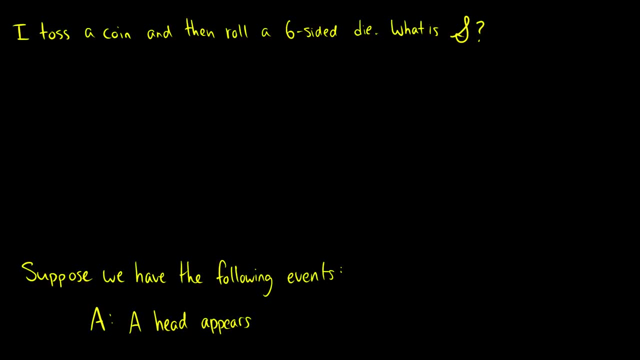 over the number of elements in the sample space. So make sure I don't have another question there. Here's another question. I toss a coin and then I roll a six-sided die. What is the sample space? Well, okay, Our first move: we can either pick heads or we can pick tails. Then, after we're going to roll a six-sided die, 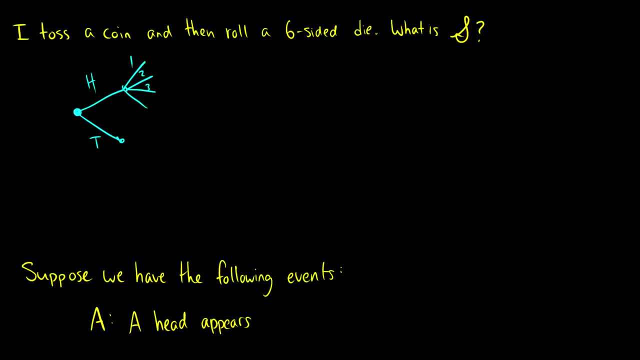 So you might pick a one, you might get a two, you might get a three, you might get a four, and so on, And same with tails. So that's the same thing Is. at the end of each of these branches we get a pair. So heads one, heads two, heads three. 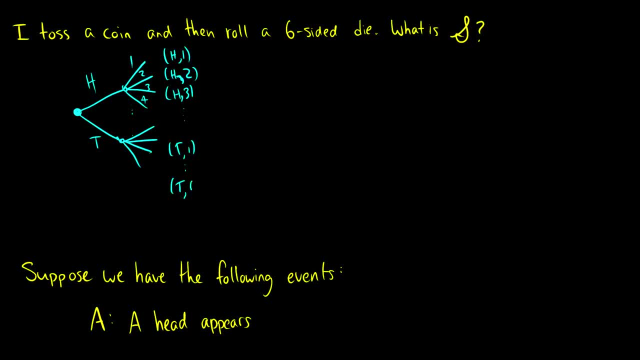 And this goes all the way down to tails one through tails six. So our sample space is going to be the set of h1, h2, and this goes all the way up to h6.. and then our next one will be tails1. 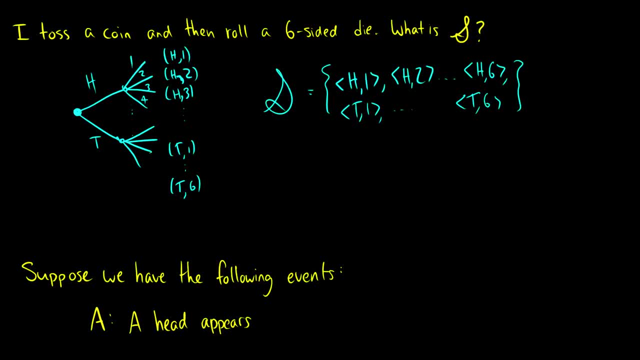 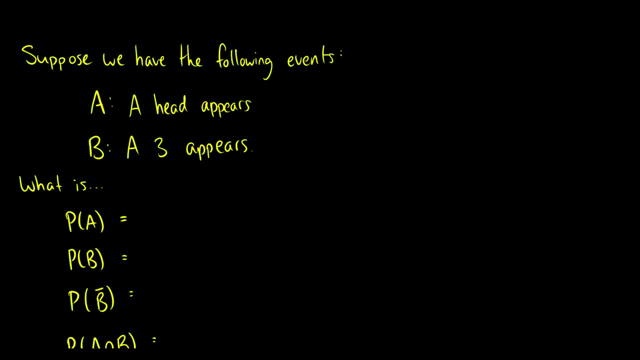 all the way up to tails6.. So our sample space has 12 elements in it. These are ordered pairs because we toss a coin and then we roll a six-sided die. So that's our sample space. Now suppose we have the following events: Event A: 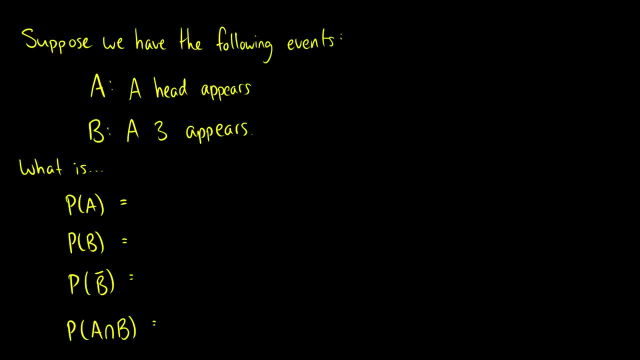 says that a head appears and event B says that the number 3 appears. So what is the probability of A happening? Well, heads occurs in 6 out of the 12 scenarios, so that's 1 half. Now a 3 appearing. this occurs in 2 out of the 12 scenarios. 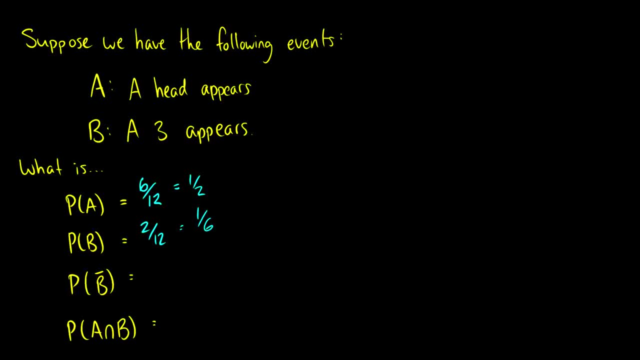 and this is going to be in 1- sixth of the scenarios, because you can't roll a number on a coin, You can only roll it on a die, And there's six possible choices on the dice, so that's a 1 in 6 chance. 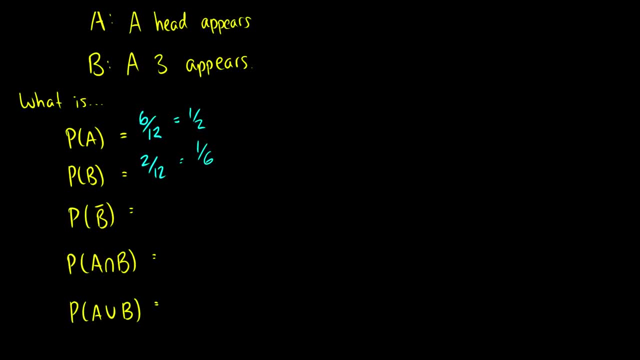 Now, what is the probability of not B? Well, this is the probability that of 1,, 2,, 4,, 5, or 6 appears, And that's going to be 5 sixths. This is also the same as 1 minus the probability of B. 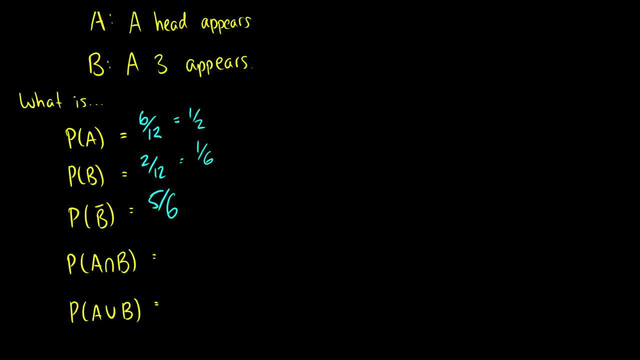 Alright, now what are the chances that both of those appears? Well, there is one scenario where a head appears and a 3 appears, And there's 12 total scenarios, so that's 1 twelfth. Now what about if a head appears or a 3 appears? 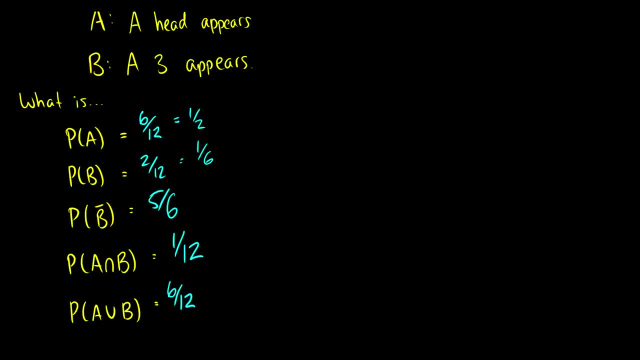 Well, there's 6 in 12 scenarios where a head appears, And then there's 2 in 12 scenarios where a 3 appears. But what happened was we counted the scenario where a where there's a head and a 3, so we have to subtract that scenario. So, really, 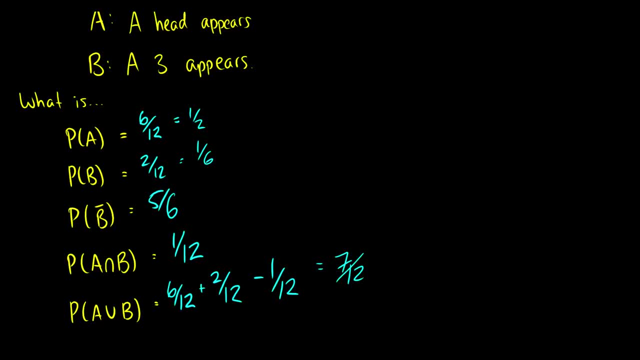 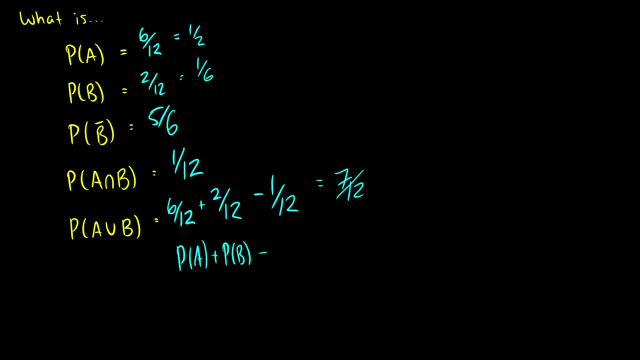 there's 7 twelfths chance that A or B happens. So this is PA plus PB, minus the probability of A and B. Okay, so you're thinking why, And I'm going to explain this again in the next video, but I think it's good to do this now too. So if we 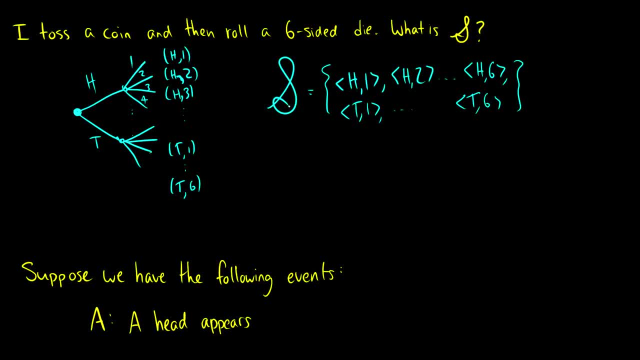 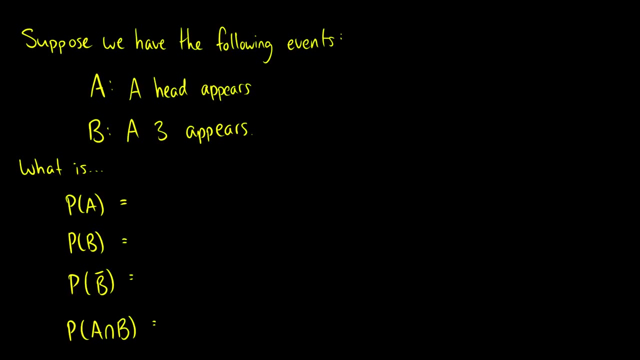 So our sample space has 12 elements in it. These are ordered pairs because we toss a coin and then we roll a 6-sided die. So that's our sample space. Now suppose we have the following events. Event A says that a head appears. 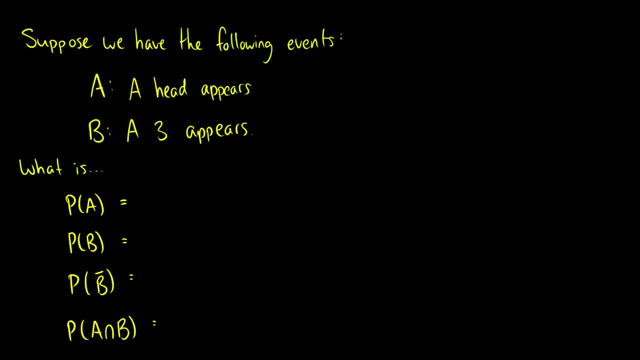 And event B says that the number 3 appears. So what is the probability of A happening? Well, heads occurs in 6 out of the 12 scenarios, So that's 1 half. Now a 3 appearing. this occurs in 2 out of the 12 scenarios. 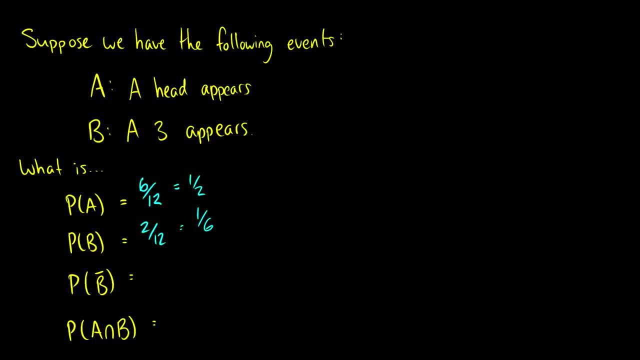 And this is going to be in 1 sixth of the scenarios, Because you can't roll a number on a coin, You can only roll it on a die, And there's 6 possible choices on the dice, So that's a 1 in 6 chance. 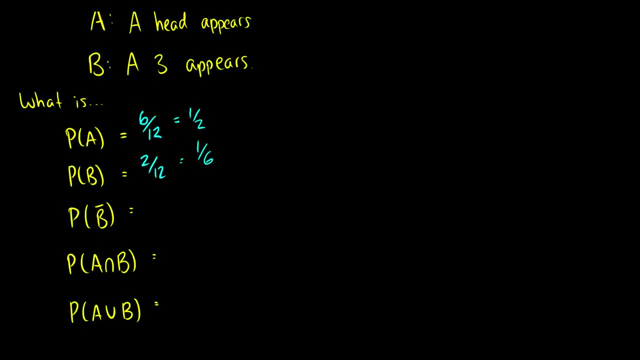 Now, what is the probability of not B? Well, this is the probability that a, 1,, 2,, 4,, 5, or 6 appears, And that's going to be 5 sixths. This is also the same as 1 minus the probability of B. 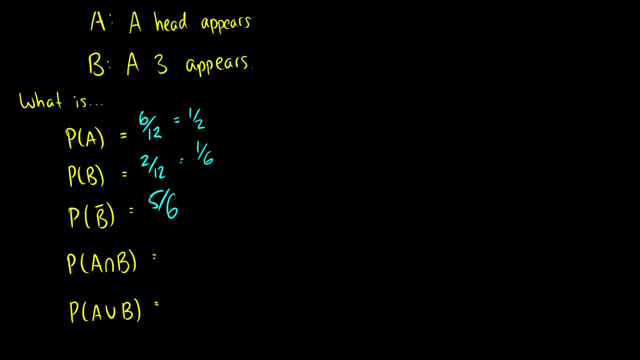 Alright, now what are the chances that both of those appears? Well, there's only one scenario where a head appears and a 3 appears, And there's 12 total scenarios, So that's 1 twelfth. Now what about if a head appears or a 3 appears? 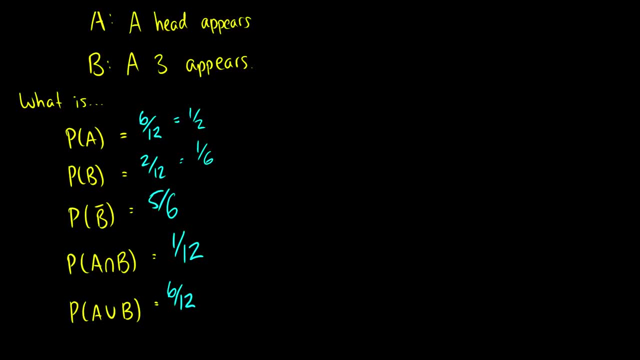 Well, there's 6 in 12 scenarios where a head appears, And then there's 2 in 12 scenarios where a 3 appears. But what happened was we counted the scenario where there's a head and a 3.. So we have to subtract that scenario. 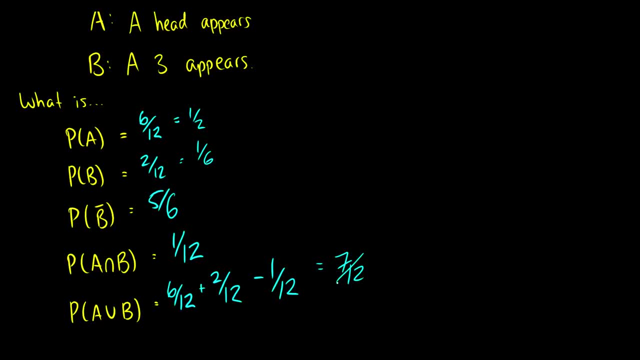 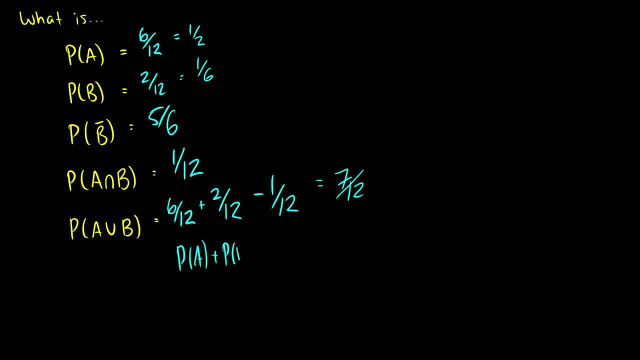 So really, there's 7 twelfths chance that A or B happens. So this is PA plus PB, minus the probability of A and B. Okay, so you're thinking why, And I'm going to explain this again in the next video. 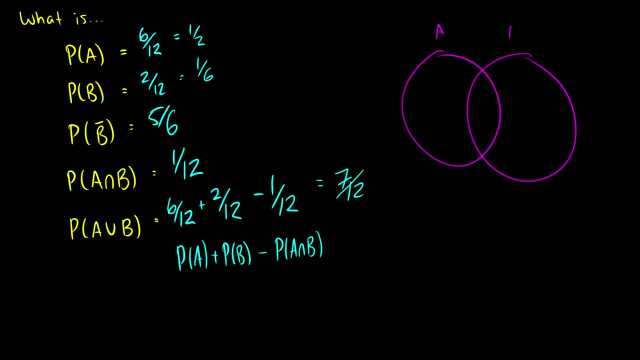 But I think it's good to do this now too. So we have an event A and B. So this is our heads here. This is our head And this is our 3.. Well, we know that in this whole bubble here, there's 6.. 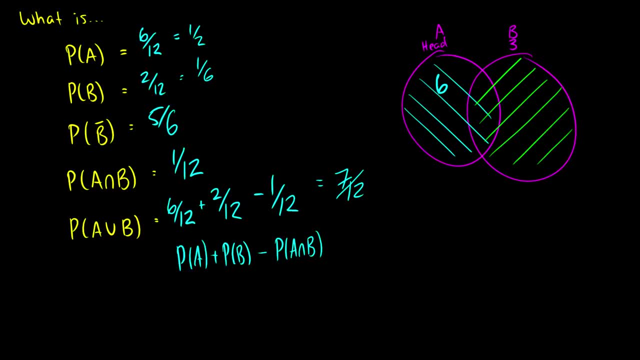 And we know that in the whole bubble of there being a 3, there's 2 scenarios where this happens. There's when there's an H and a 3, and a tails and a 3.. And in this head we have H1, H2, all the way to H6. 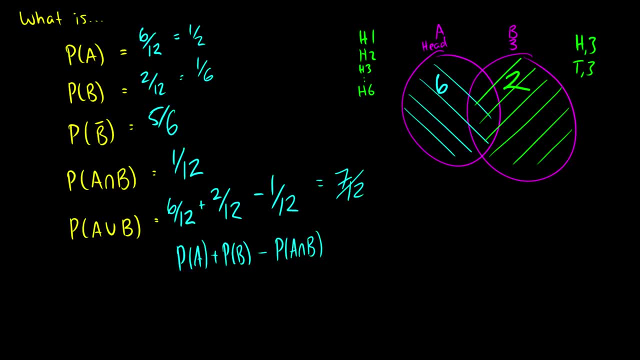 In fact I'm going to include H3 in here, But this overlapping area here has H3 in there. But the problem is that we counted H3 once in the heads and we counted H3 once in the 3s, So we've counted it twice. 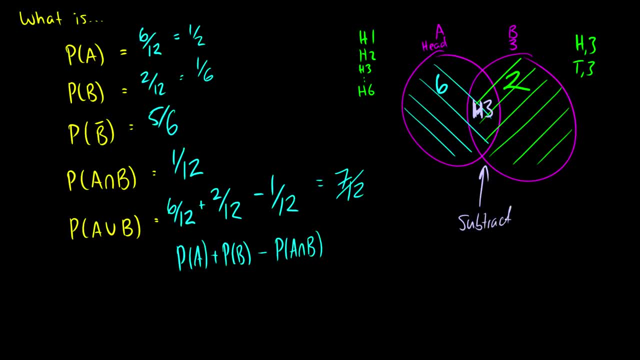 So what we have to do is we have to subtract the number of times H3 occurs or that both events happen. So we have to remove this area, because we've counted it twice already. So then when we remove it, we have the total number. 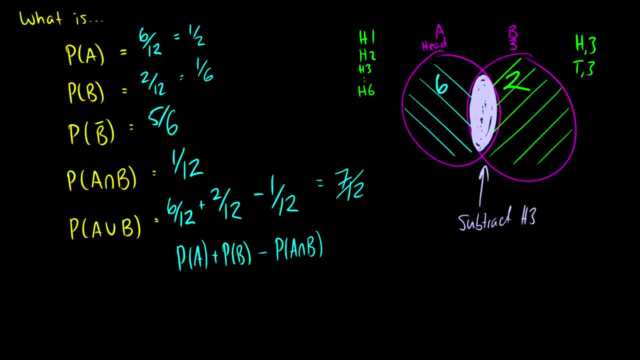 So that would be 7 twelfths. So that's basic probability. Questions can be more difficult than this a little bit, But the main part of the course is not about this basic stuff. It's about axiomatic probability, which I'll cover next time. 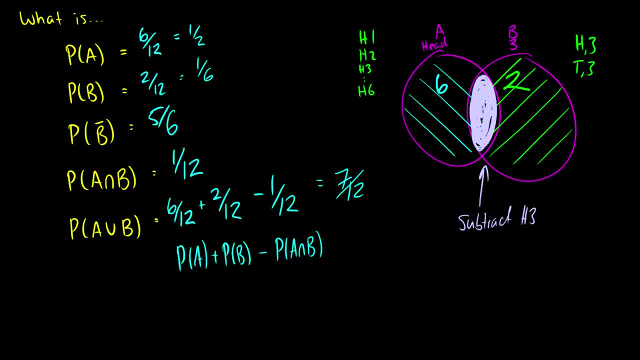 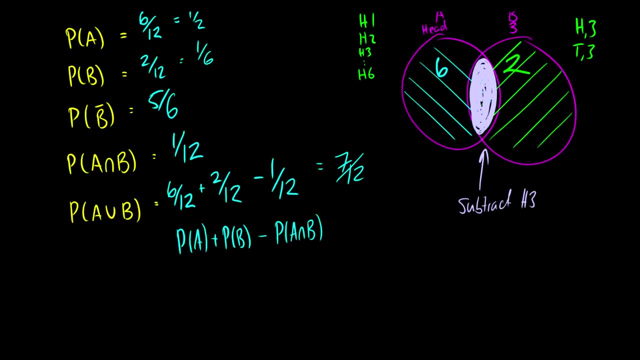 and conditional probability, which will take a couple videos to explain because that's a little bit more challenging. So, as always, if you have any questions, leave them in the comments below. If you want to see more of this stuff, you can check out. 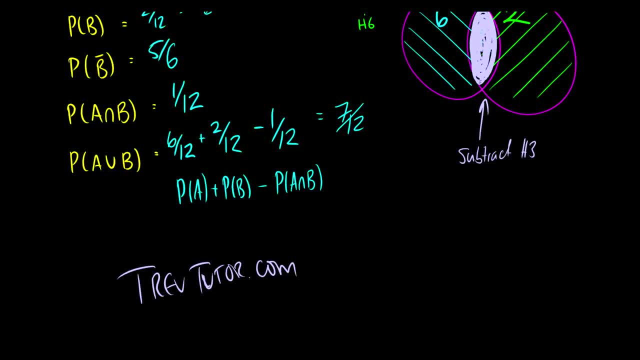 trevtutorcom and there's exams videos, other courses on there And if you really enjoy this stuff, share it with your friends. It's always great to be passed around as that guy on YouTube that teaches you stuff. So thanks for watching. have a great day. 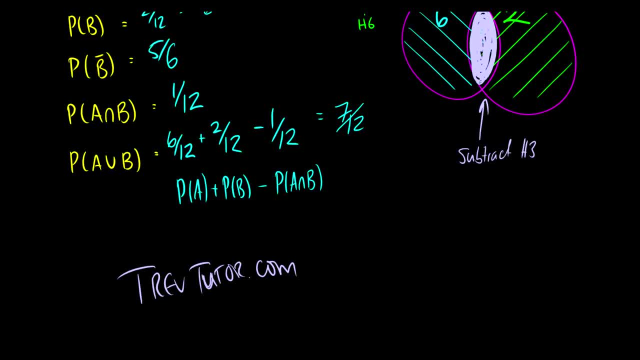 and hopefully I'll see you for some axiomatic probability next time, because that stuff's fun. The first big challenge in discrete mathematic proofs. It's going to be fun. 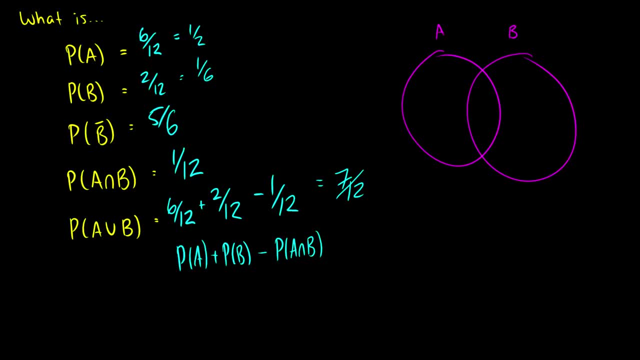 have an event A and B. So this is our heads here and this is our 3.. Well, we know that in this whole bubble here there is 6, and we know that in the whole bubble of there being a 3, there's 2 scenarios where this: 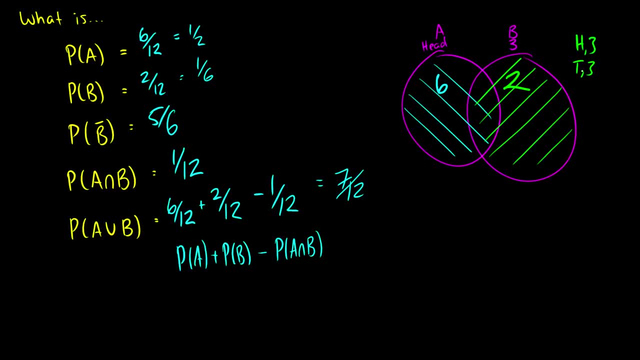 happens There is when there's an H and a 3, and a tails and a 3.. And in this head we have H1, H2, all the way to H6. In fact, I'm going to include H3 in here, But this overlapping area here. 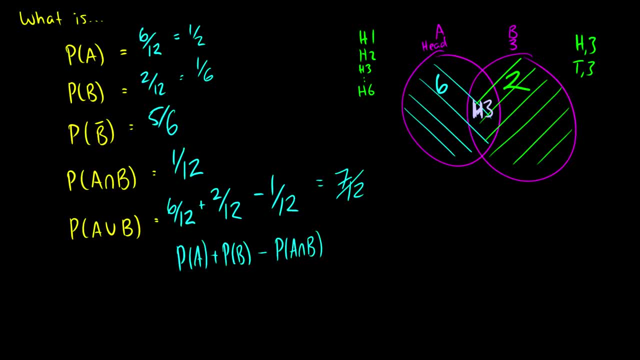 has H3 in there, But the problem is that we counted H3 once in the heads and we counted H3 once in the 3s, So we've counted it twice. So what we have to do is we have to subtract the number of times H3 occurs or that both events happen. So we have to remove this area. 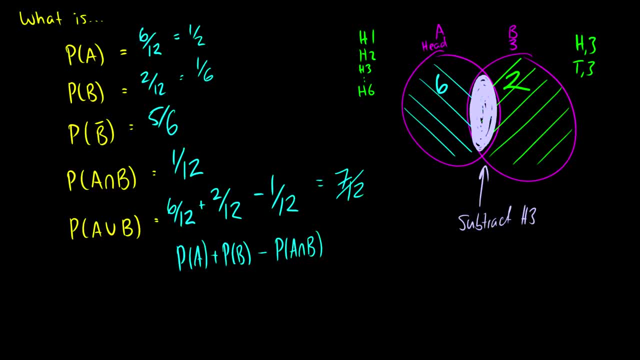 because we've counted it twice already. So then when we remove it we have the total number. So that would be 7 twelfths. So that's basic probability. Questions can be more difficult. This a little bit, But the main part of the course is not about basic stuff. It's about 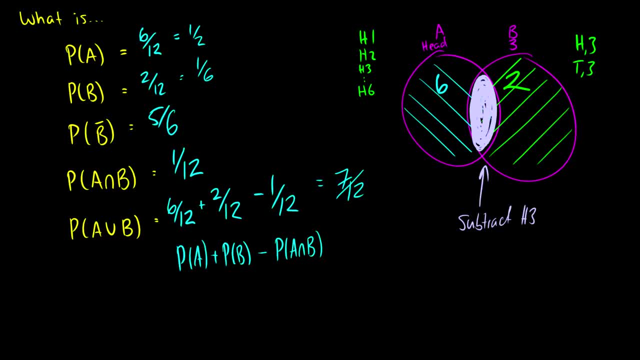 axiomatic probability, which I'll cover next time, and conditional probability, which will take a couple videos to explain, because that's a little bit more challenging. So, as always, if you have any questions, leave them in the comments below If you want to see more of. 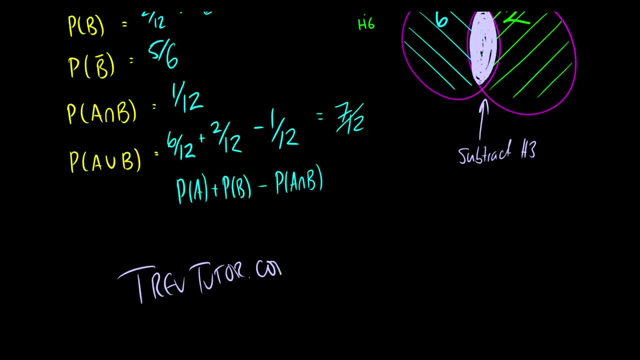 this stuff. you can check out trevtutorcom And there's exams videos, other courses on there And if you really enjoy this stuff, share it with your friends. It's always great to be passed around as that guy on YouTube. 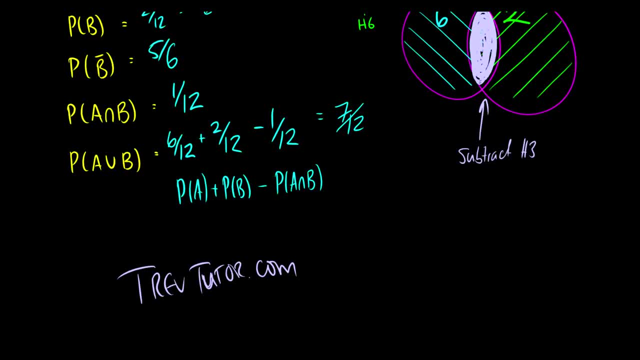 that teaches you stuff. So thanks for watching, Have a great day and hopefully I'll see you for some axiomatic probability next time, because that stuff's fun. The first big challenge in discrete mathematic proofs is going to be fun.